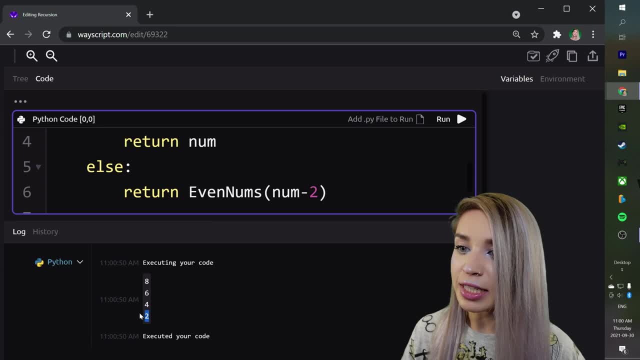 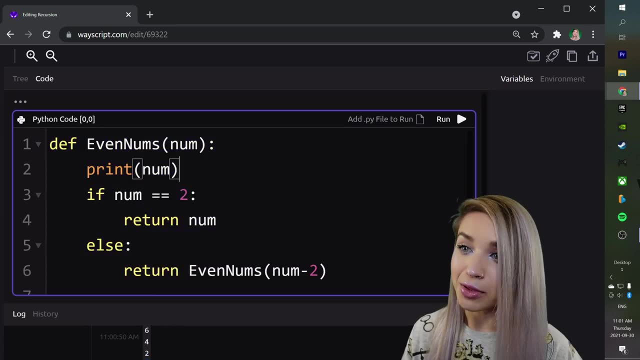 So it looks like we're getting the results we've expected, where our base case is printed last. But we can always go the extra mile and we can tackle odd numbers as well. So if num modulo two doesn't have the remainder of zero, And in this case we would like to print a message of, please, 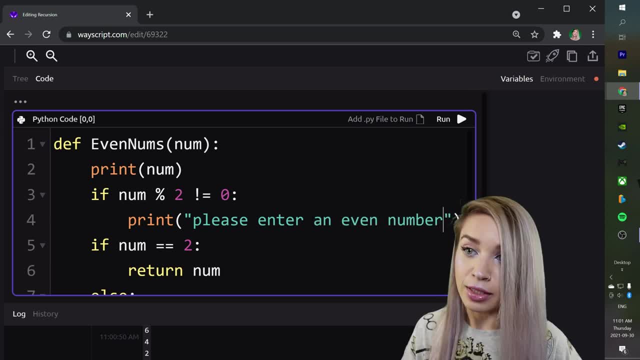 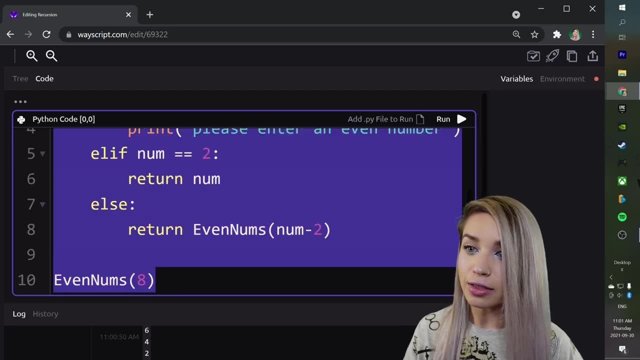 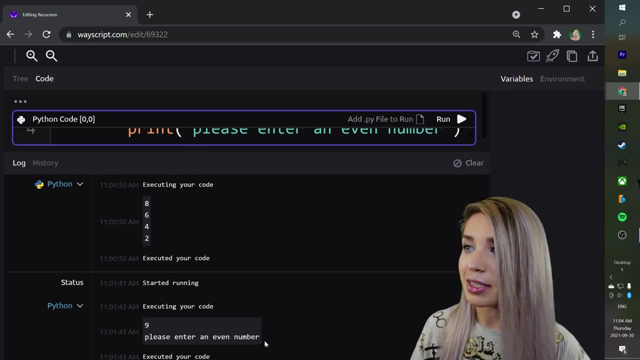 be a number and even number, And then, additionally, we will turn this if statement into an else if statement. And now, even if we call this function on an odd number, let's say nine, and we run this code, And then, instead of getting an error, we're simply getting a message to improve. 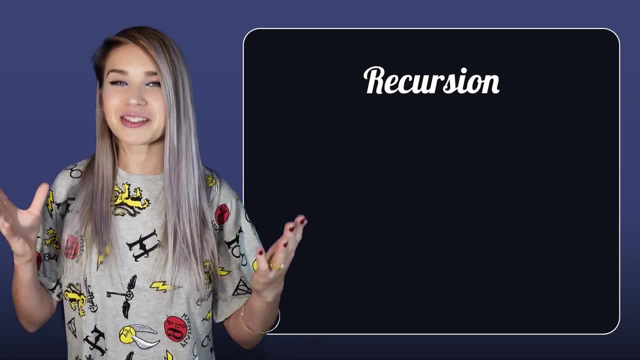 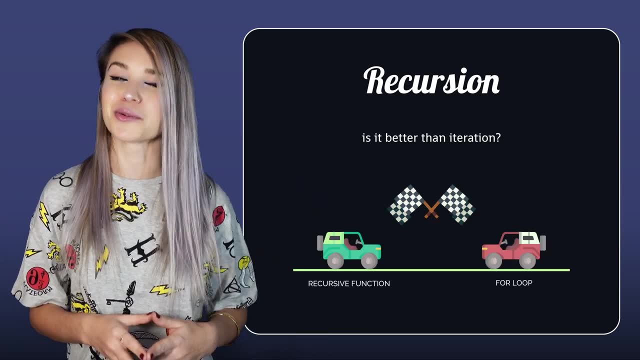 our input. Cool, So we've seen how recursive functions work, But are they really better than for loops? For this we will look at another code example using the feedback function we just created using the Fibonacci sequence. Now, Fibonacci numbers are a very special sequence. 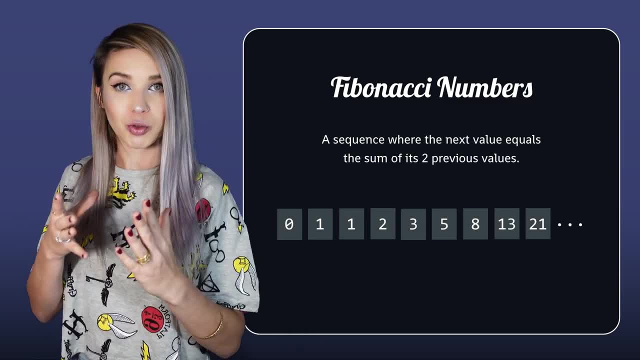 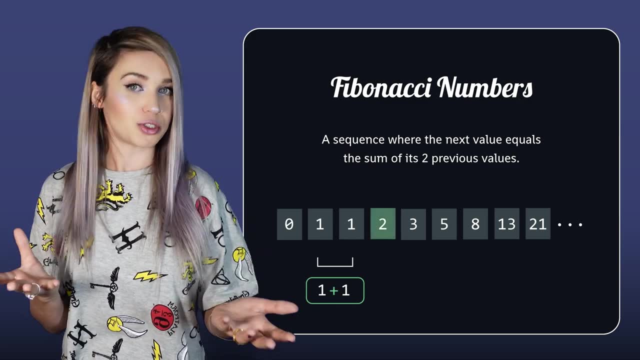 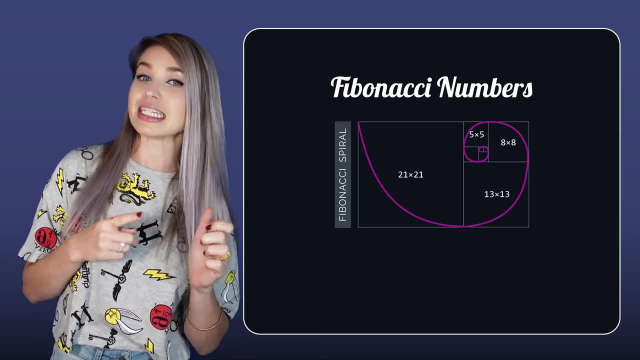 where the next value always equals the sum of its two previous values. So, for example, zero plus one equals one, one plus one equals two, one plus two equals three, and so on until infinity. We can find this sequence in nature in Pascal's triangle in sacred geometry. 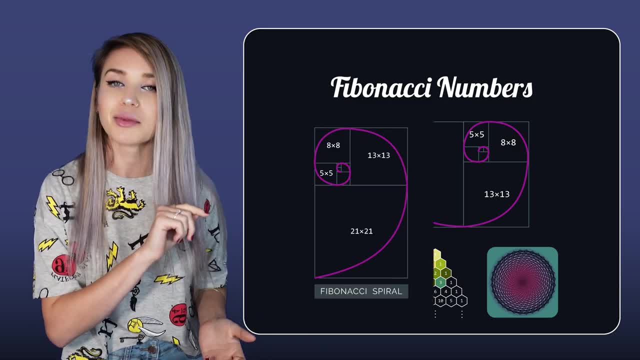 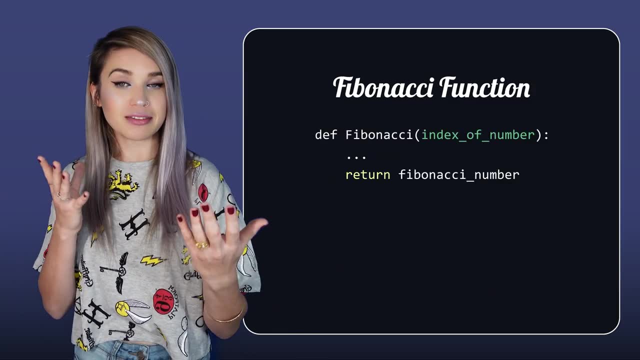 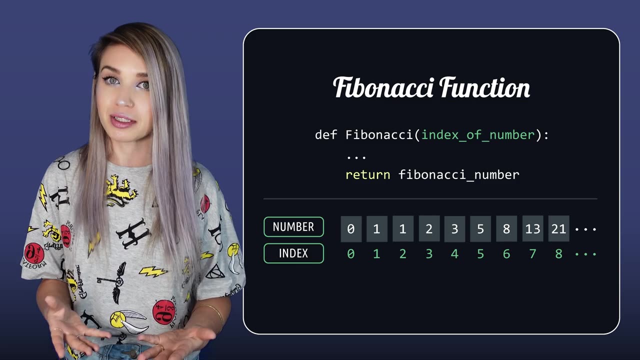 and pretty much anywhere we look, including the Mona Lisa. But how exactly do we compute it? Let's consider a function that takes in a positive numeric value. This value represents the index of the Fibonacci number. we want to return, So, for example, at index zero. 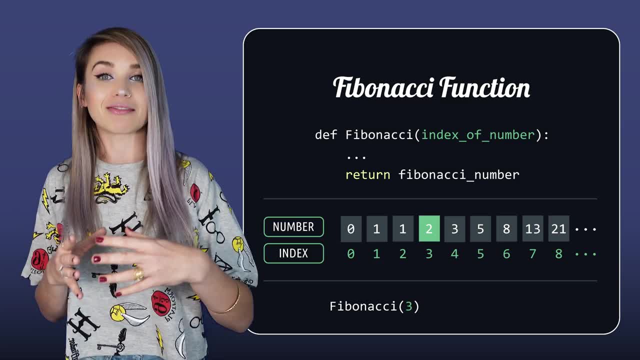 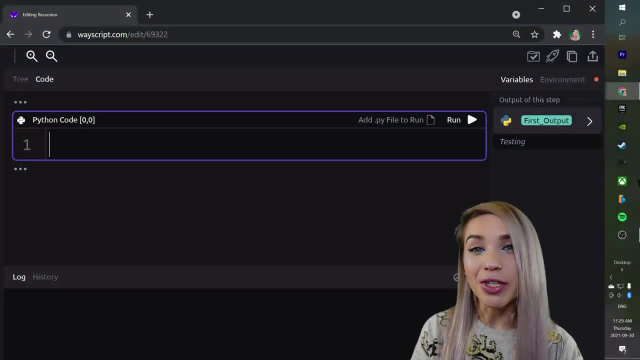 we have the number zero At index three, we have the number two At index eight, we have the number 21, and so on, And we will begin. We will begin with the recursive function and we will call it Fibonacci with a capital F. 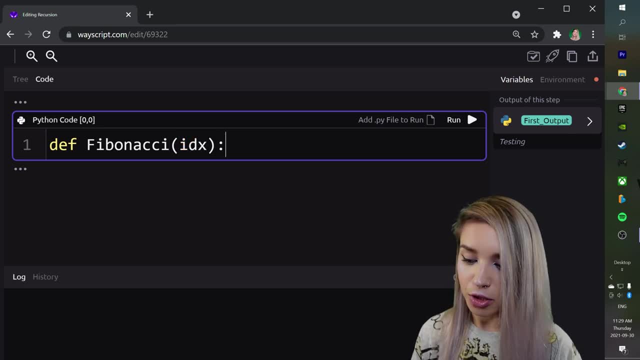 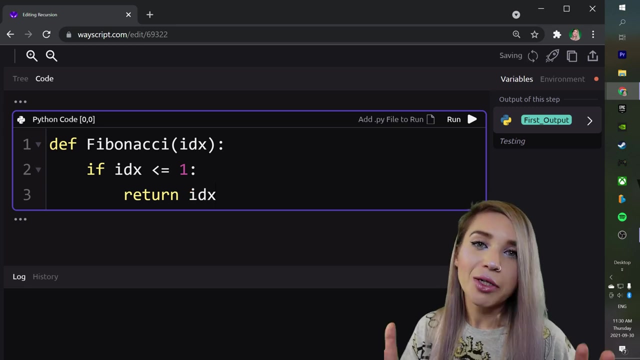 We can then pass an index value of our choice to this function And, as usual, we will tackle the base case first. Now, if our index is either smaller or equal to one, we will then simply return the index itself, which is exactly what we've done in our previous example. 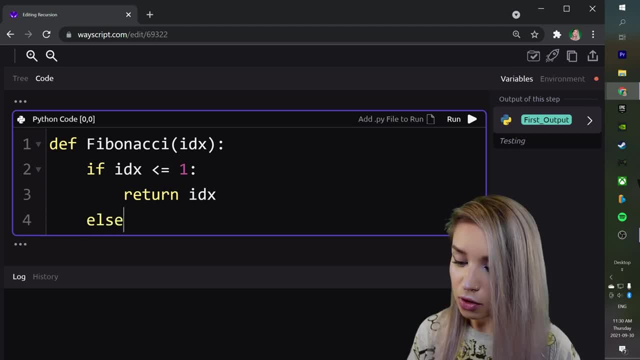 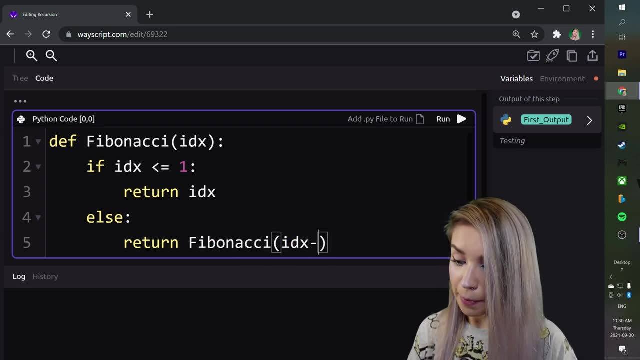 However, if this is not the case, inside our else clause, we will return an instance of our Fibonacci function call where we pass our index minus one, And then this takes care of the previous value. Now, additionally, we will add another instance. 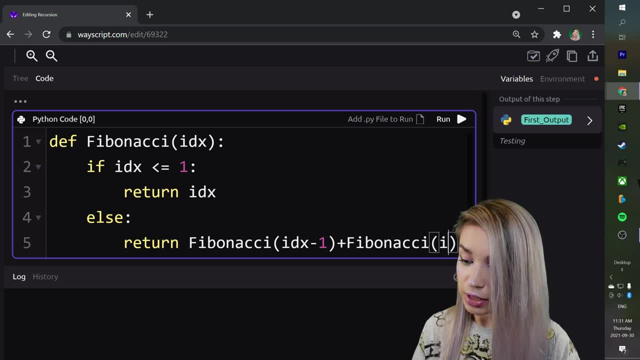 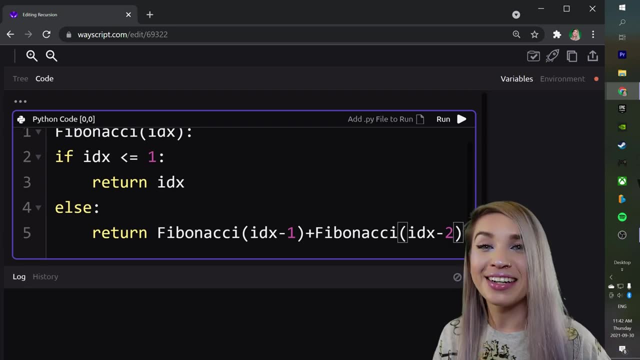 of the Fibonacci function, but this time we will pass it on index minus two And of course my head is probably blocking it. And surprise, surprise, our function is complete. Now let's go ahead and check if it works. So at the bottom we have our index. 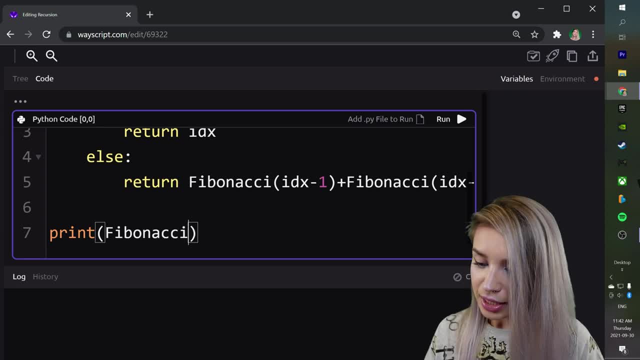 At the bottom, we will print an instance of Fibonacci And, at least at first, we will check it on index zero. Now, as you guys have seen before, this should return the number zero. Perfect, we are getting zero in return. 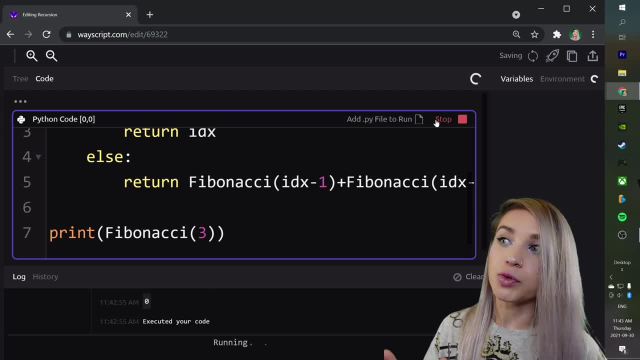 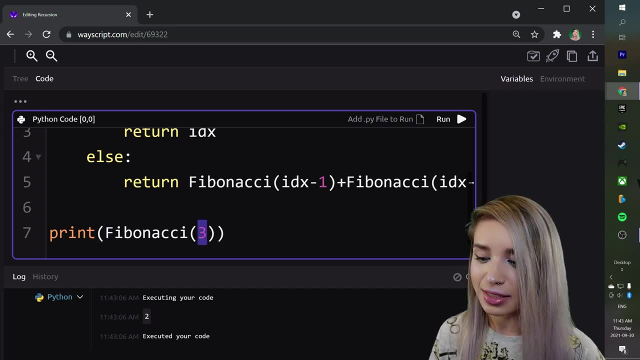 So let's boost it to index three. This should return the number two. Perfect. and just to be extra cautious, let's also call it on the index eight, And this should return 21.. Ah, perfect, Perfecto, bravo. 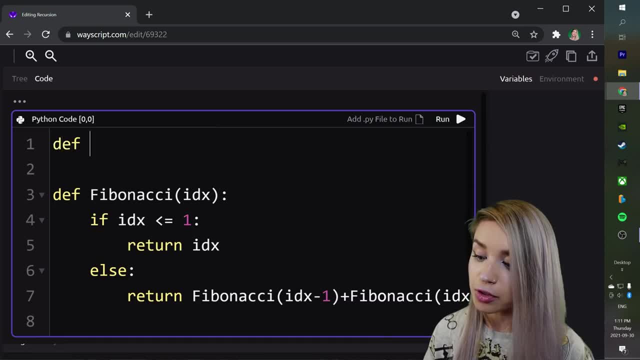 Now, in terms of iteration, we will define a brand new function called Fibonacci, with a lowercase f. this time We will also pass an index value to this function, but in order to start looping, we need to account for the first pair of Fibonacci numbers. 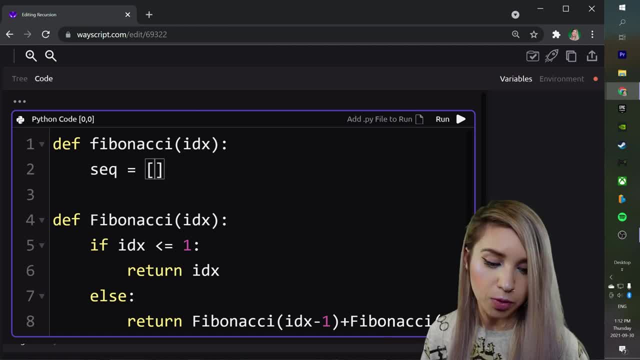 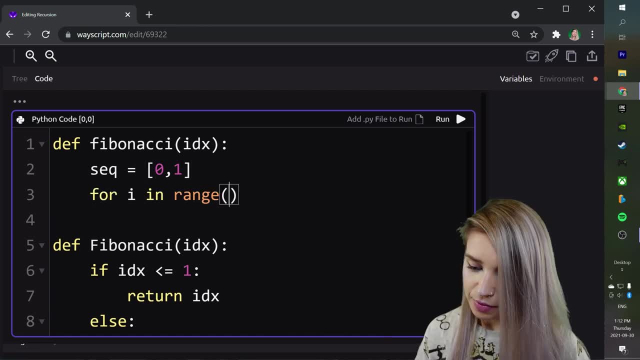 We will call this pair sequence and we will assign it to a list with zero and one, And now we can go ahead and start looping. So for i, in range index, zero and one, And then for index we will append a brand new value. 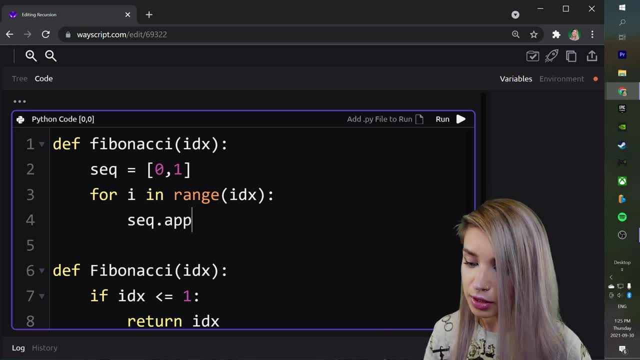 to our sequence. So we will type sequenceappend where the value would be the sum of the last item in our sequence represented by index minus one, plus the item in our second last sequence represented by minus two, And then we can go ahead and exit the for loop. 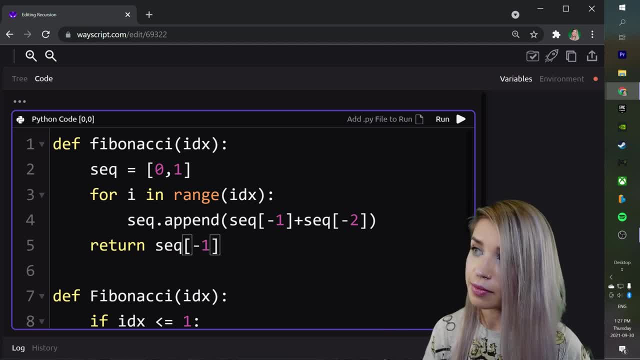 and we will return sequence in the index of minus one, But note that since we have a number zero, we will return. and we will return sequence in the index of minus one, But note that, since we have a number zero, Since we've started with two values rather than one, 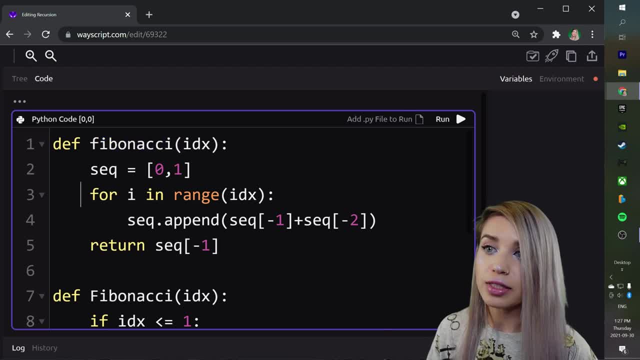 if we will call Fibonacci on index zero, it will skip this for loop altogether and we'll return the last value of our sequence, which is one, while we're actually looking for zero. So the way to fix it is quite simple: Instead of returning the last value, 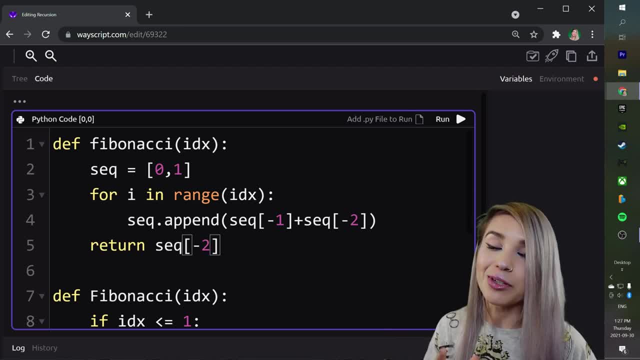 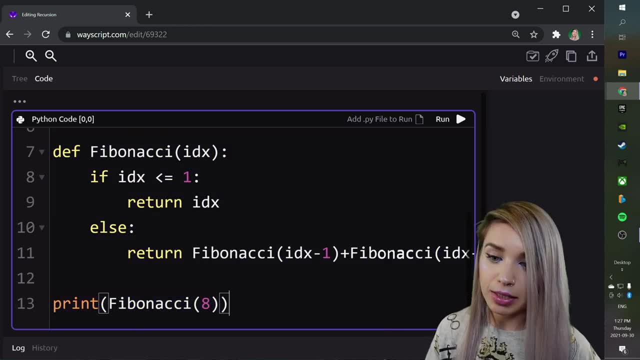 we will simply return the second last value. And now our iteration function is complete. Let's go ahead and call it. at the very bottom, We will simply copy this print statement statement and we will refactor the capital F to a lowercase f. Let's go ahead and run this script. 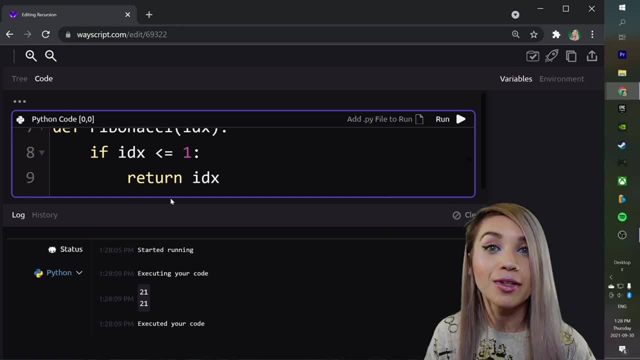 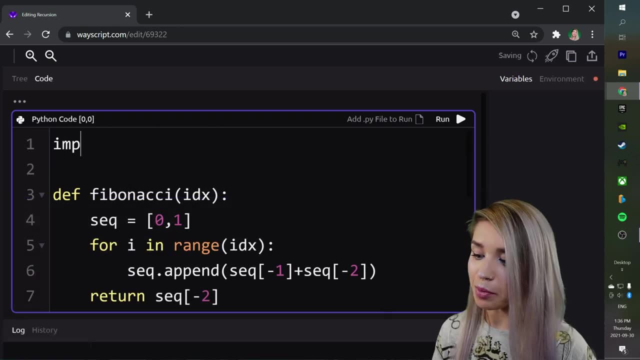 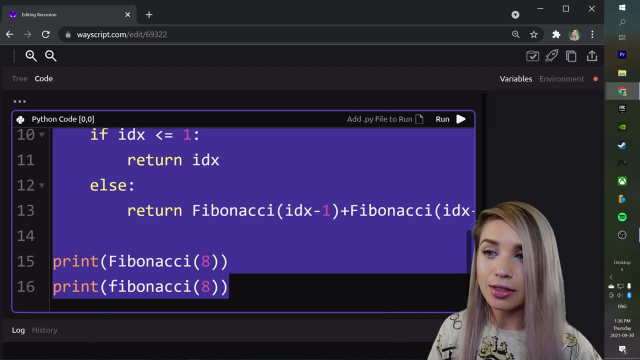 Beautiful. So both our functions return the same value, the correct value. but then how do we know which one of these is more efficient? For this we will first import the time module, and then we can record the time that takes for both our functions to run. So, right above our function calls, we will. 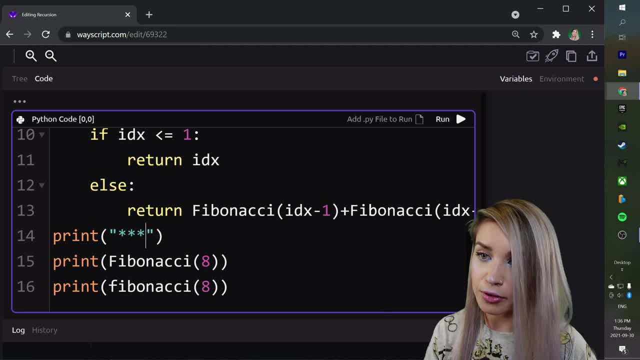 type the kind of function we're dealing with. In the first case that would be recursion, and right before we call it we will record the current time with timetime. We can then assign it to a variable called rec and then, right after our function call, we will print an additional statement. 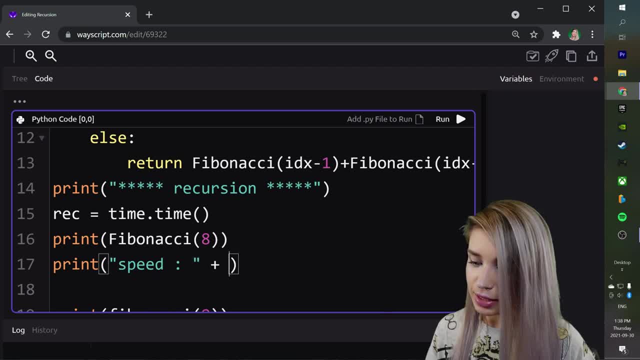 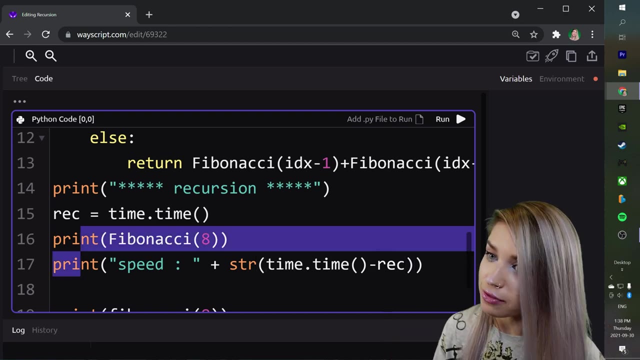 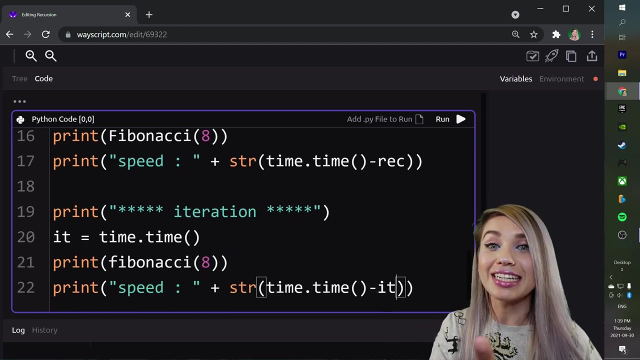 speed to which we will concatenate the string instance of the current time with the current time minus the time we have recorded earlier inside a variable called rec, And we will, of course, do the same for our iteration function. Cool, Now let's run it and find out once and for all which is. 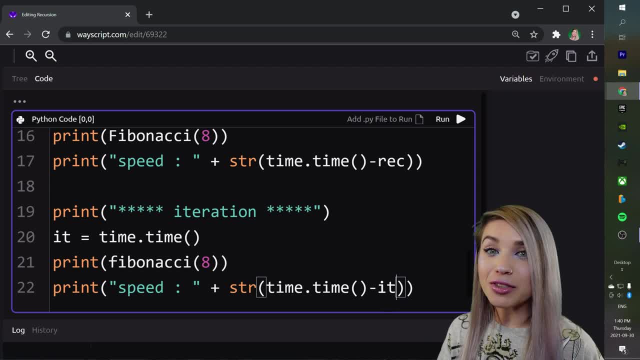 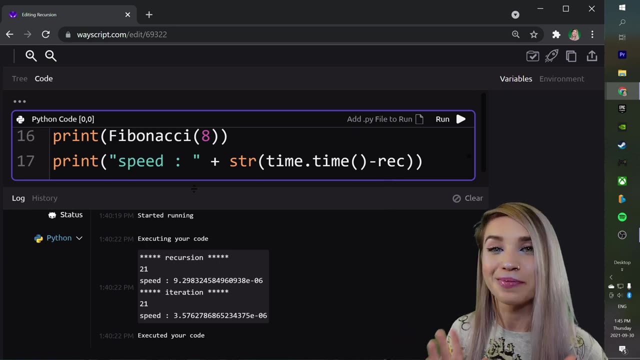 faster: iteration or recursion? And before we do this, I want you guys to make a guess and then we will see if it turned out. So let's go ahead and click on run, And if your guess was iteration, you got it, because it is actually twice as fast as recursion. 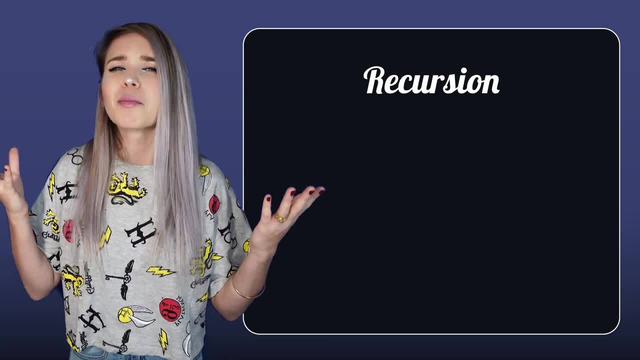 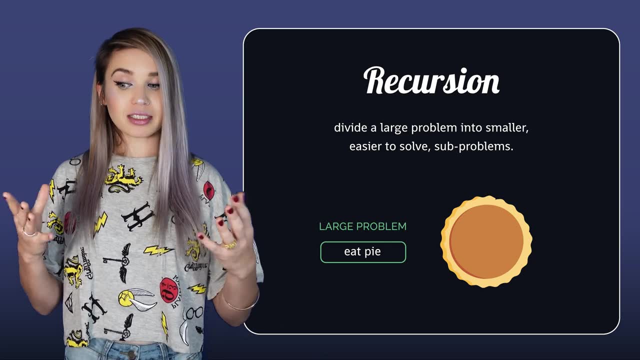 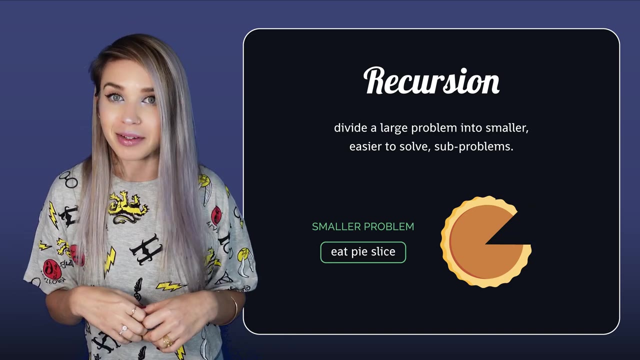 Good job. So why it is so important to us, then? Recursion is a very basic computer science concept. It helps us divide a very big problem into smaller sub-problems which we can easily solve one at a time. We call this process divide and conquer, and you guys will encounter it a lot in.